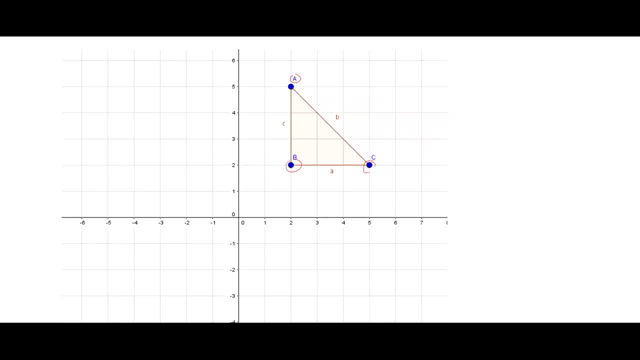 Right Now on the graph here we have, this is the x-axis, And let me tell you from now, if that is the x-axis, it is also: the line y is equal to zero. Right, Some people do not grasp that concept, But the x-axis is the line y, equal to zero. 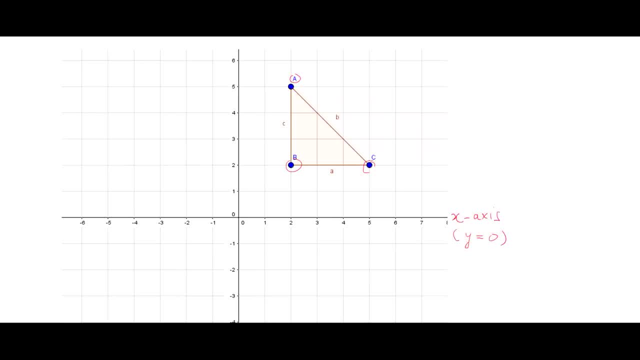 So if they ask you what is the equation of the x-axis, it's: y equals zero, The vertical axis Is the y-axis Right And y-axis is also the line x is equal to zero. Now, a long time ago, when I know started doing this, what I used to remember is that if it's the x-axis, then it's reverse. 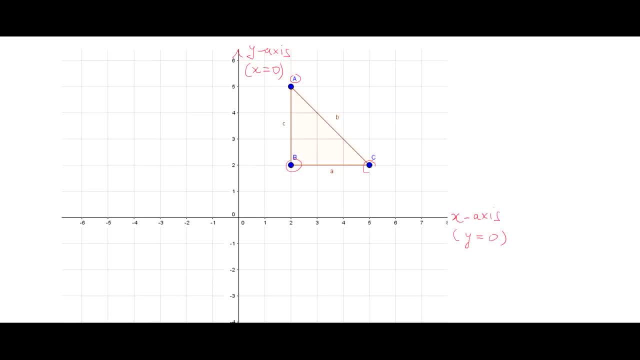 It's the line y equals zero. If it's the y-axis, then it's reversed: It's the line x, equal to zero. OK, so what we're going to do, we're going to perform a reflection on this triangle. So whenever you have to do a reflection, the 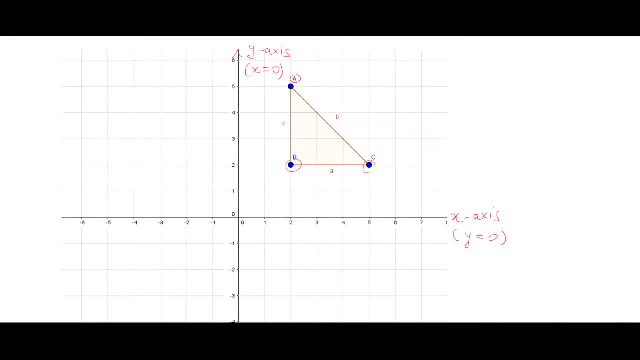 Whenever you have to do a reflection, the You need to indicate what the mirror line is Right. So we are going to use the y-axis as our mirror line Right, Or the line x equals zero. So therefore we're going to perform a reflection. 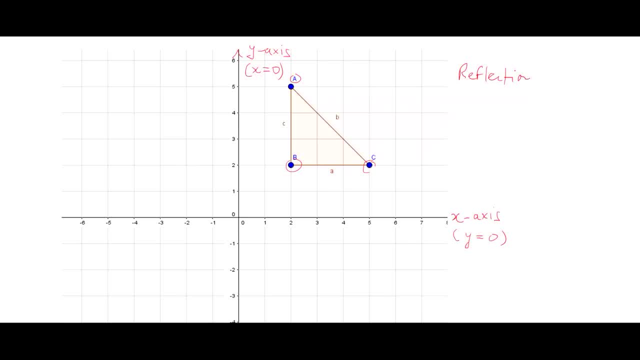 So it's a reflection Reflection In the y-axis or the line x equal to zero. Right Now, this is what we use to describe a reflection Right. You have to give the mirror line. So if the y-axis is a mirror line, 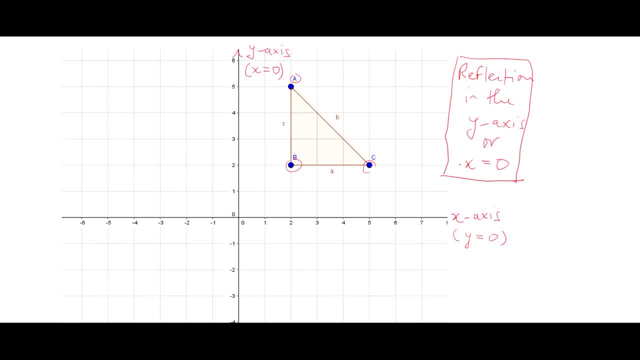 Now this is a point. here We look at the distance of E from the mirror line. So we see that from here to here We have one, two units, so we have to go two units behind the mirror. So therefore, this point here will be E prime, which is the image of E. 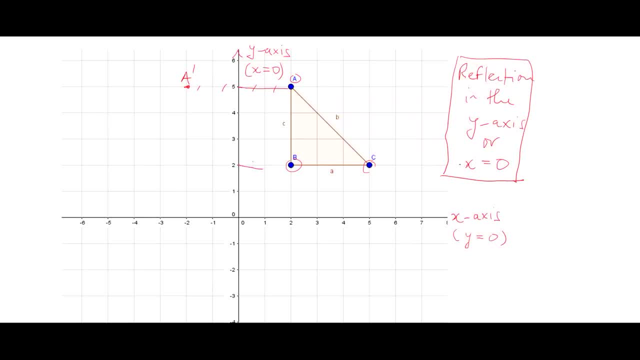 Then, in the case of B, We draw a line from the point B to the mirror line. We have two units, So therefore we go one, two units behind the mirror line. So therefore this is B prime. In the case of C, 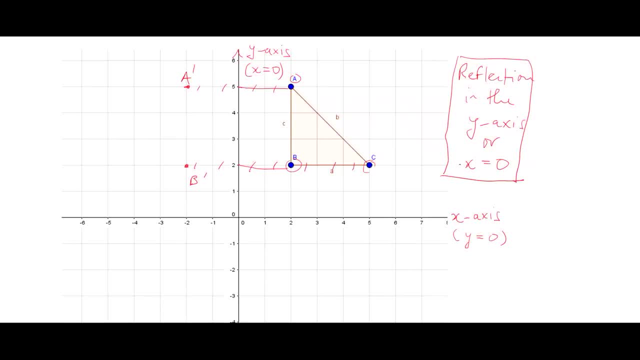 We have One, Two, Three, four, five, So we have to count five units behind the mirror line. So we go one, two, three, four, five, And this is C prime, the image of C. So therefore, our triangle now is: 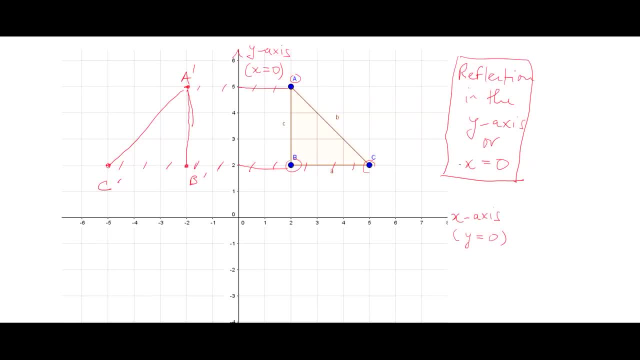 sorry, so this is our image right Now. if you notice something, the triangle, this is the object, right, And this is the image. If you notice something, the triangles have the same size, the same shape. however, they are mirror images of each other, right, But the two triangles. 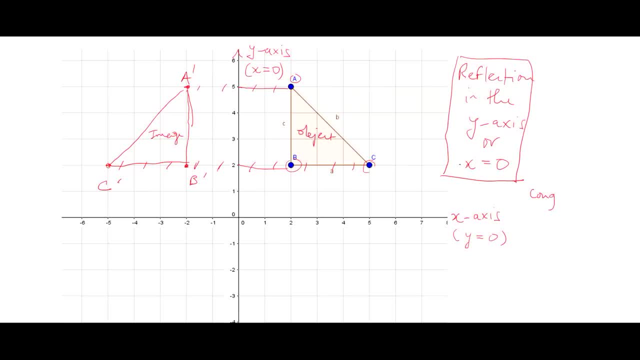 are said to be congruent. right, This is a term that you're going to meet a lot when you're doing transformational geometry. So the two triangles are said to be congruent. Their angles are the same, Their lengths are the same, because the length A- B is the same. 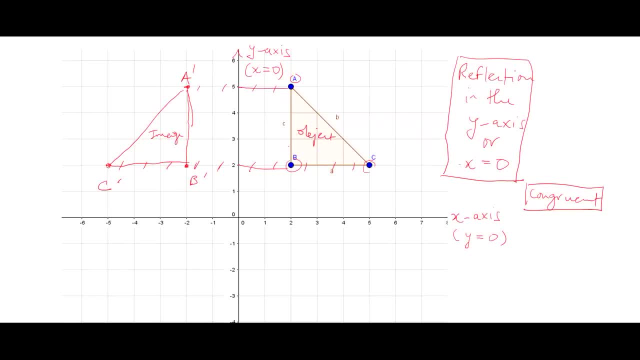 as the length A prime, B prime. The length B, C is the same as B prime, C prime. So the triangles are congruent, right? This is something that they ask you and they expect that you say: that the object and the image are congruent, right. 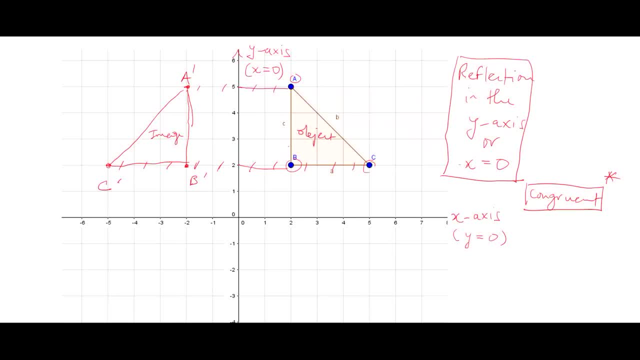 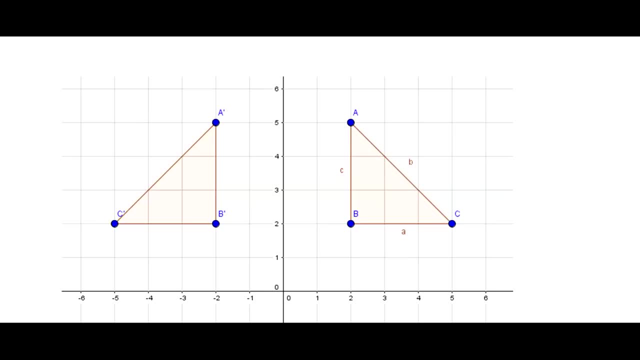 What else do you need to know here? Okay, so, alright, so this is the solution, basically. So we are doing a reflection and the line X equals to zero, or my Y axis, right? So this is my object and this is my image. 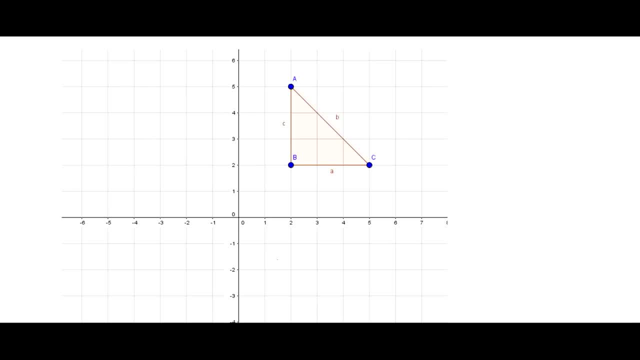 okay, Now let's do another one. In this case I am going to do: we have a triangle again and let's label our axes. So this is our X axis, or the line Y equals to zero. This is our Y axis. 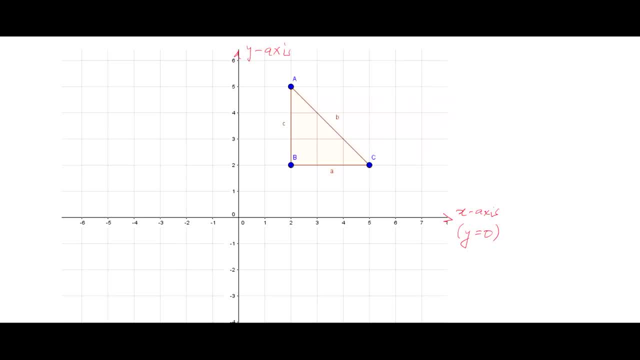 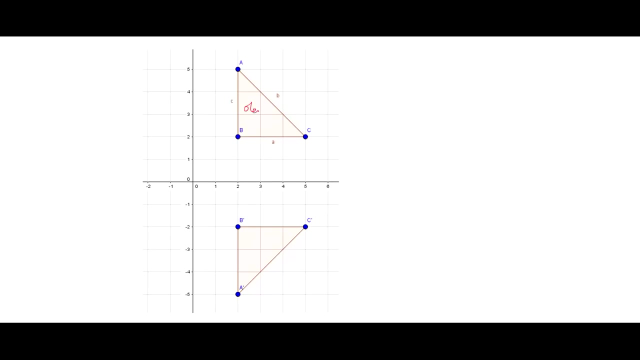 or the line x is equal to 0. So we want to do our reflection here. So let's hold on. I don't have enough space here, so let me use the final answer. So this was our object, which is a triangle. 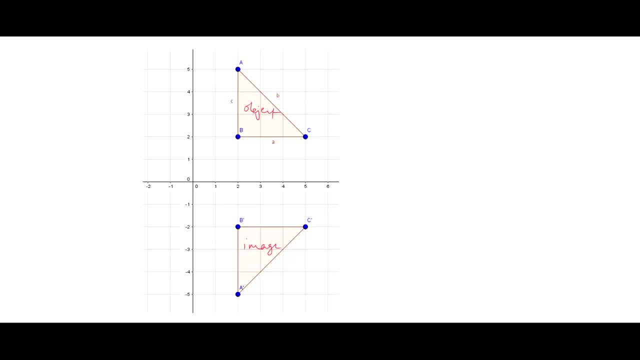 This is our image, this is the line, this is your x-axis, or the line y equal to 0.. Alright, so if you notice the point, let's say b is one, two units from your mirror line and the point b prime is two units behind the mirror line. 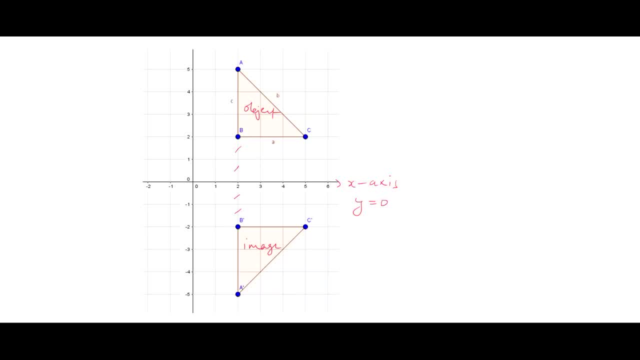 The same thing for c. Alright, we have one, two units here. we have one, two units here. in the case of a, you have one, two, three, four, five. so we go one, two, three, four, five units behind the mirror line. 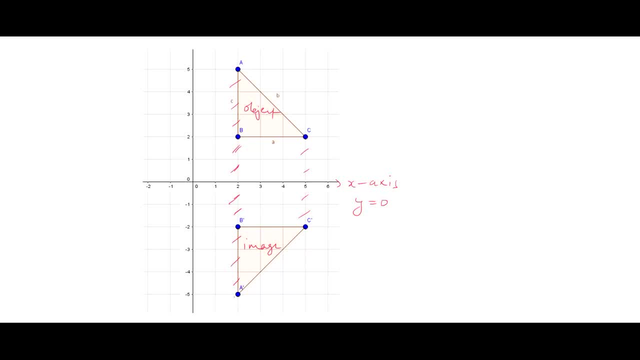 and that's how we get e. Alright. now they can give you a diagram like this and they can ask you: what is the transformation Now? to identify a reflection? the object and the image will have the same size. the lengths will be the same. What will be different is that 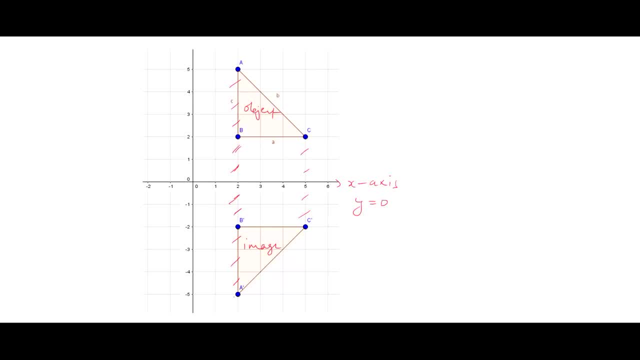 the image looks flipped, So they are mirror images of each other. So if this was on a piece of paper and I were to fold the paper along the x-axis, the two images- the object and the image- will coincide, meaning that the point a will line up to a prime. 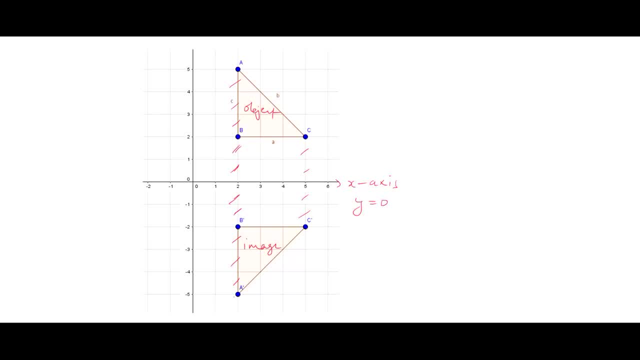 b will line up with b prime and c will line up with c prime. Alright, that is if I fold it along the x-axis or the line y equal to 0.. Now in a question, they will ask you to identify the transformation. You might have to describe it. 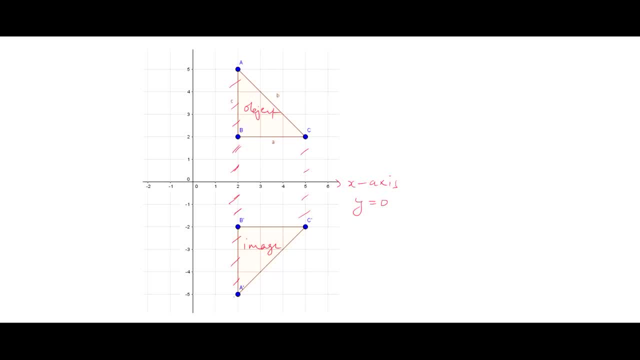 If it's a reflection, you need to state what the mirror line is, and then you need to state what the mirror line is. The mirror line in this case is y, equal to 0. And you could be asked to construct a line to show where the mirror line is. 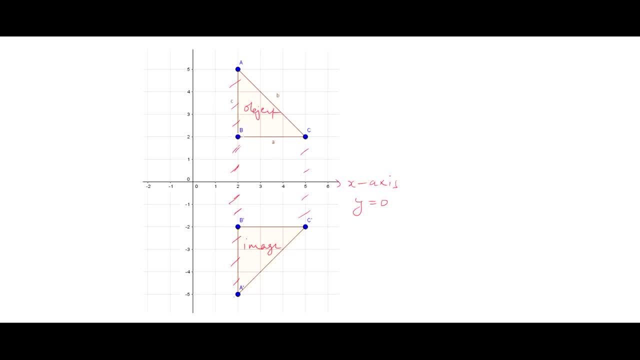 All you need to do, if you know it's a reflection. let's say you draw a straight line between b and b, prime and what you do. you use your compass and you draw some construction lines. So you start at, let's say, point b and you draw. 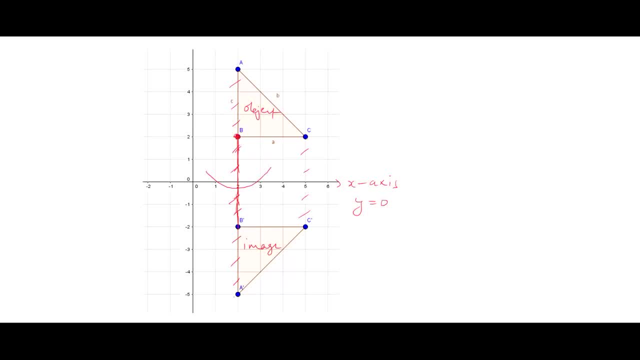 something like: you draw an arc here and, using that same arc, you're going to draw another, another arc here, and then we draw this line here, which is our mirror line. So, really and truly, the mirror line will be the perpendicular bisector of b, b prime. 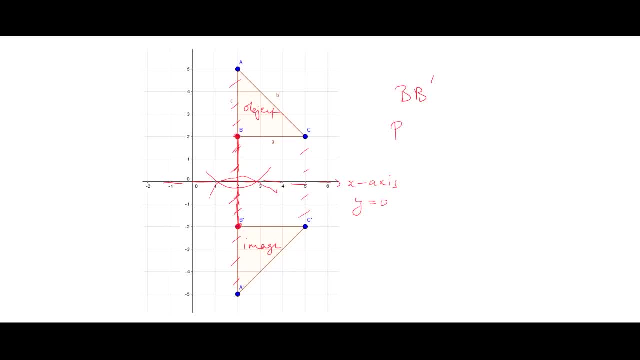 So the line b, b, prime, if we find the perpendicular bisector, will be the mirror line, Right. So a perpendicular bisector is just a line that divides a line segment into two equal parts. right. So the line segment here is b. 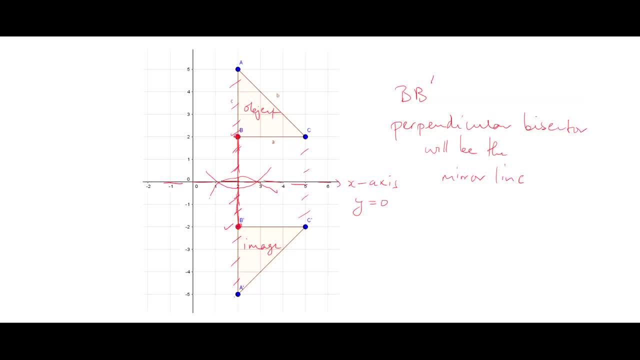 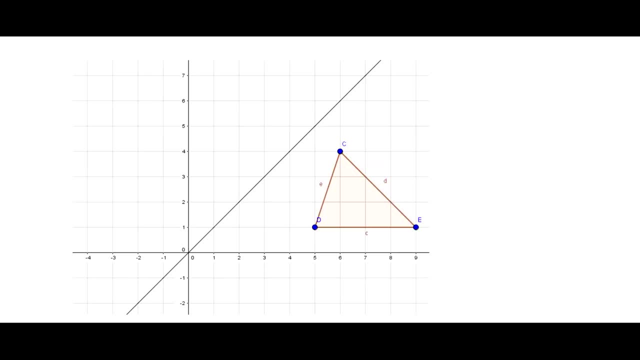 b b prime. So the perpendicular bisector of b b prime is really my mirror line. Okay, So let's do another one. here We have, let's leave a little axis. We have the x-axis, We have. 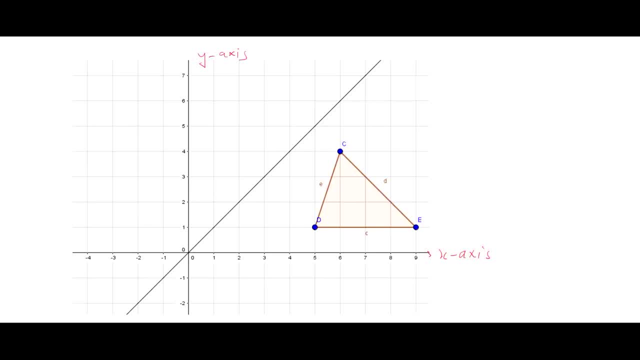 the y-axis. So the x-axis is the line y equal to zero And the y-axis is the line x equal to zero, And I've drawn a line here which is y is equal to x And I'm going to perform a reflection of this triangle here. 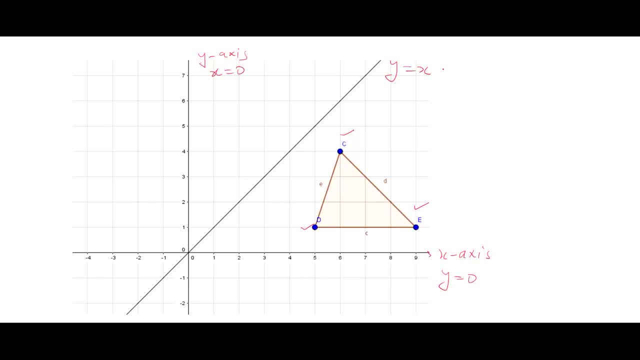 which is c, d and e, And I have to show what happens Now. the angle is the mirror line. So this is our mirror line, right? Some students get confused here now because they're not. they're not sure what to do. 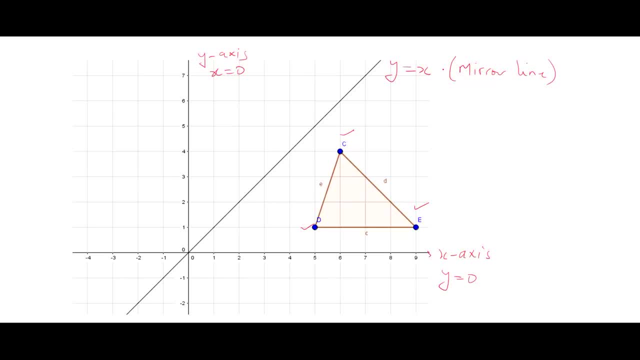 Alright. What you have to do is to draw a line. Let's say you want to find the coordinates of c prime. You have to draw a perpendicular line- This is our perpendicular line here- That's 90 degrees To your mirror line, and then extend it. 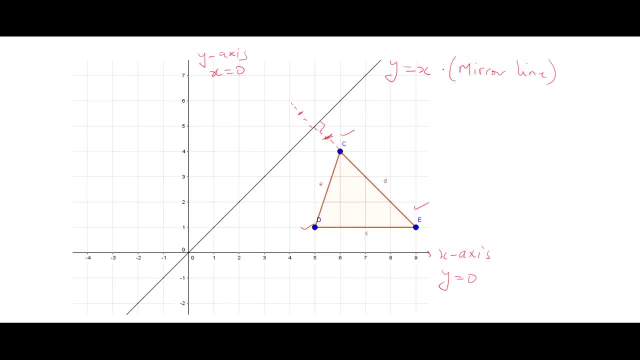 So this distance here right has to be the same as this distance here. So therefore this point will be c prime. In the case of d, you have to do the same thing again. You draw a line that is perpendicular to the mirror line and you have to measure this distance here. 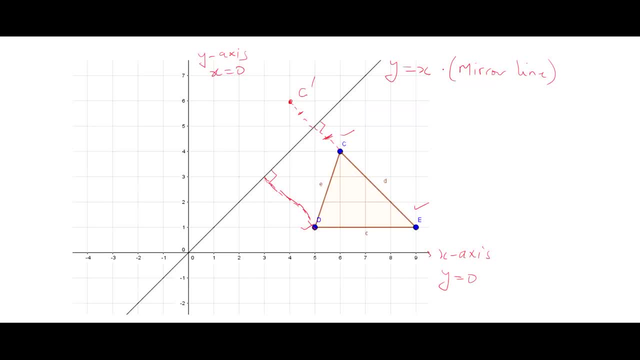 That is this distance here. Measure this distance, and we go that same distance behind the mirror line right Now. I'm just sketching here, so this could be slightly of the solution in the next slide. right, And you do the same thing for e. 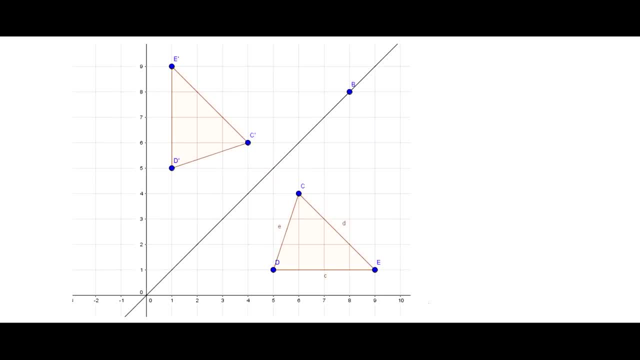 So the solution really will look like this, right? So this is our line, y equal to x, which is our mirror line, and this is our object and this is our image, right? So cc prime, you notice, this line here is 90 degrees, and the same thing for d as well. 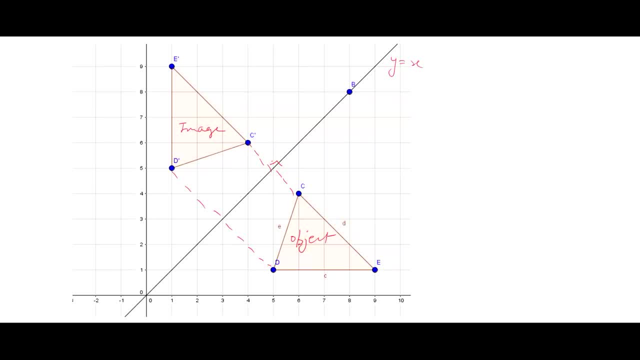 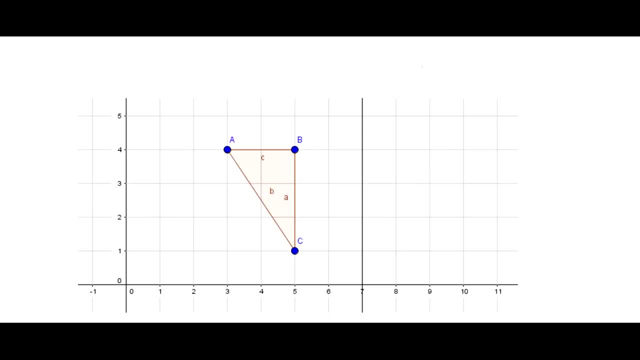 OK, so reflections are pretty straightforward. um, let's do one last one. okay, so we have a triangle: a, b and c. this is our x axis and i'm going to say it again, it's also the line y is equal to zero. this is our y axis, and it's also the line x equal to. 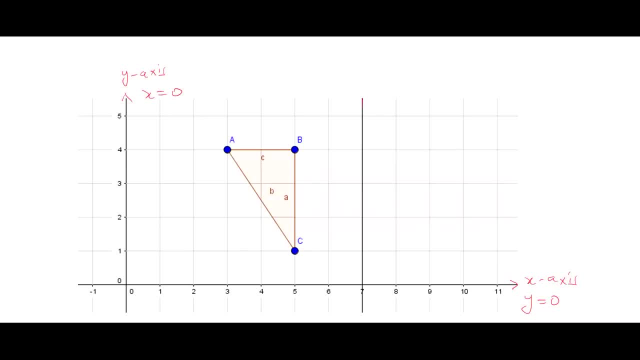 zero, this line that we have here, this vertical line here, right, it's the line x equal to seven, right? why is it the line x equal to seven? this is our x axis here, right, this is our x axis, and we are counting zero, one, two, three, four, straight up to seven. so, therefore, this is the 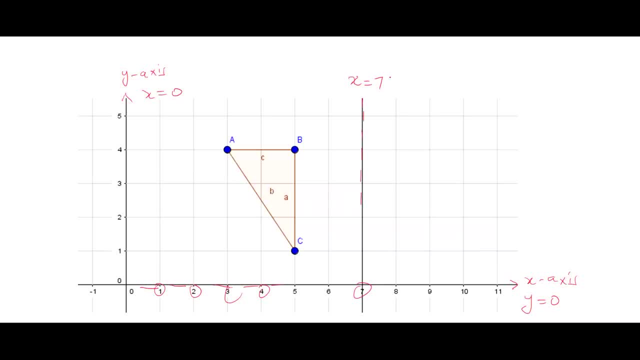 line x equal to seven. if i were to draw a horizontal line at this point here, this: the equation of that line is: y is equal to five. okay, so be careful how you label your lines. so i want to do a reflection in the line x equal to seven. 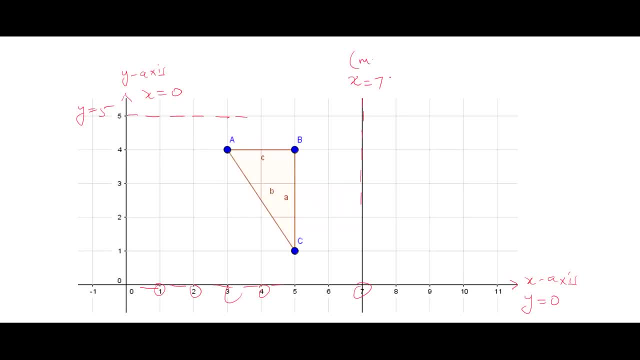 so x, x, equal to seven, is our mirror line. so this is our mirror. and let's start with b. we draw a line from b to the mirror line, which is 90 degrees. we measure this distance here. so this is one, two units. so this will be one, two units. so therefore, this point here is the point b, prime. 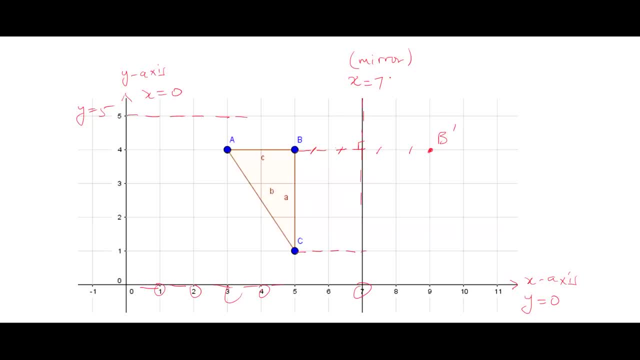 i took at c and draw a line of vertical perpendicular line to the mirror line and i measure my distance. so one, two, we go behind the mirror line. one, two. so this here is c prime. we do the same thing for e. so we draw our line going this way.